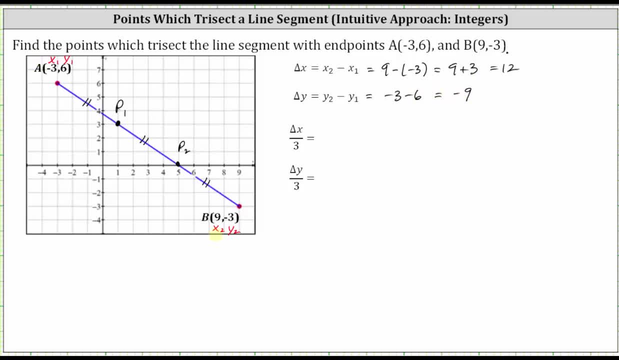 which is equal to negative nine. Y decreases by nine from point A to point B, And now we'll divide these changes by three, as we're looking for the points that trisect the line segment. The change of X divided by three is 12 divided by three. 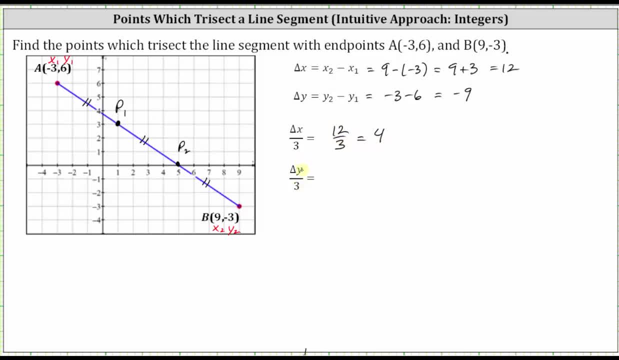 which is four. And delta Y divided by three, or the change of Y divided by three is negative nine divided by three, which is equal to negative three. So now we know the change of X is four and the change of Y is negative three. 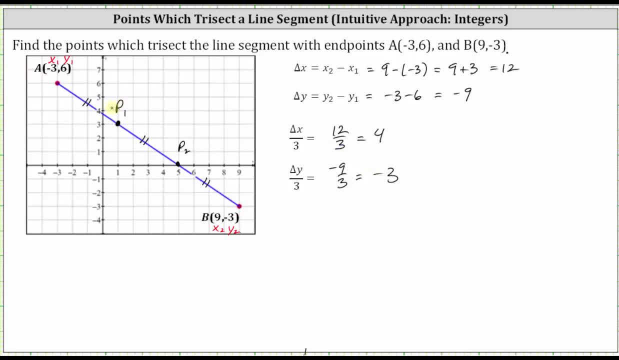 From A to P sub one, from P sub one to P sub two and from P sub two to B. To show this, starting at point A, if the change of X is four, we would go right four units, Because the change of Y is negative three. 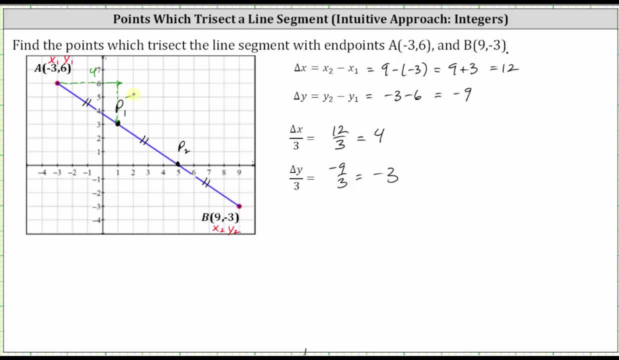 we would go down three units to find the ordered pair for P sub one, From P sub one to P sub two. we would do the same. We would go right four units because the change of X is positive four. Down three units because the change of Y is negative three. 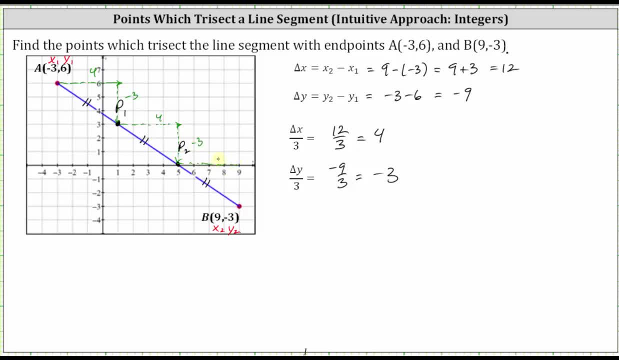 And just to verify: if we go right four and down three, again we are at the end point, point B, And now let's calculate the ordered pairs for P sub one and P sub two. To find the ordered pair for P sub one. 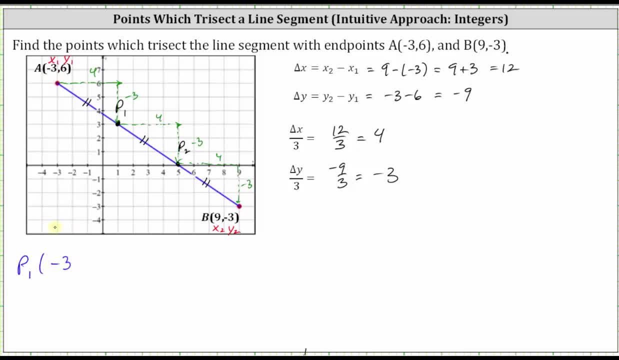 we start at point A, so X is negative three, and then add delta X divided by three, which is positive four, And the Y coordinate starts at six and then decreases by three, so we add negative three, which gives us P sub one has an X coordinate. 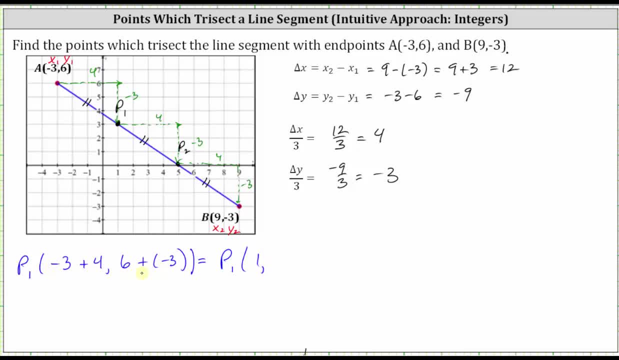 of negative three plus four positive one and a Y coordinate of six plus negative three, which is positive three. And now to find the ordered pair for P sub two, we add delta X divided by three to the X coordinate of P sub one. 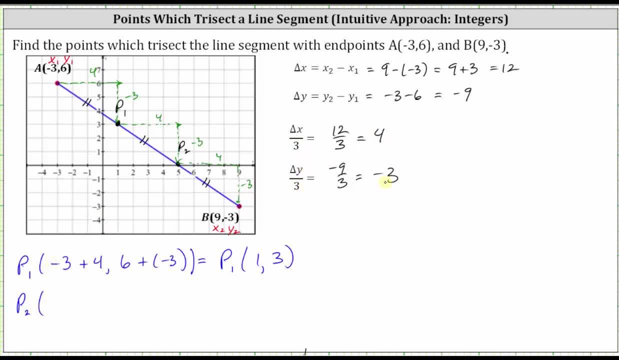 and we add delta Y divided by three or negative three to the Y coordinate of P sub one. So P sub two has an X coordinate of one plus four and a Y coordinate of three plus negative three. Simplifying the X coordinate is five.